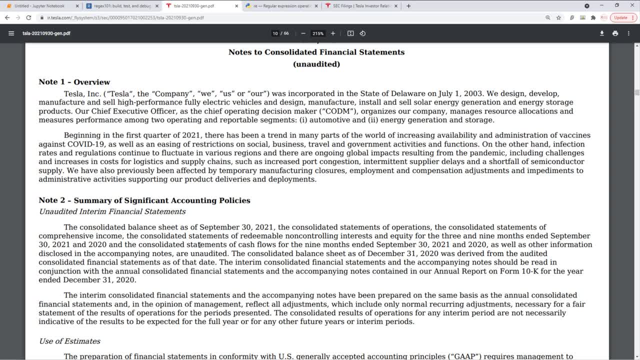 of significant accounting policies. let's say you are a python engineer and you you have already used OCR to extract this text from this document and now you're using regular expression to get the titles. you know these two titles, so that's your end goal. we are going to open regex101.com. 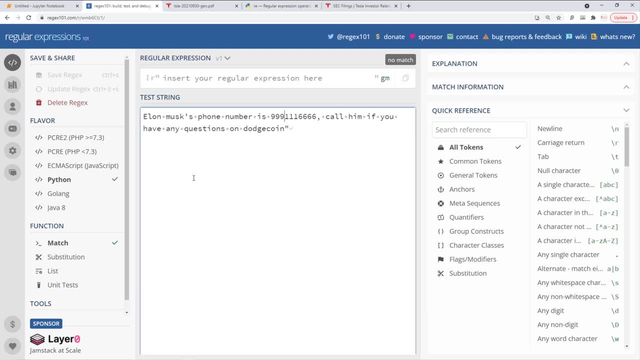 which is an amazing website that I love. personally, I use it all the time to build my regular expression here first, and then I use that in my code. this is short of like a test pad that you can use it all the time. again. I'm using this website all the time here on the right hand side. 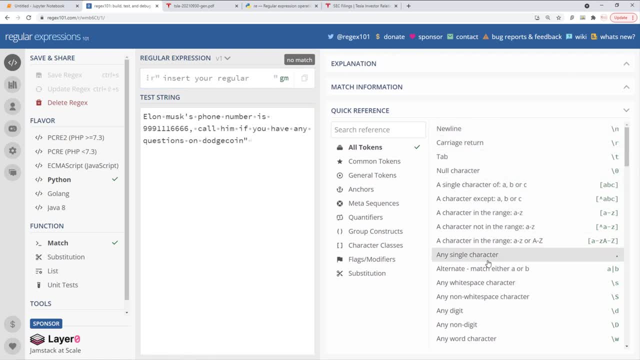 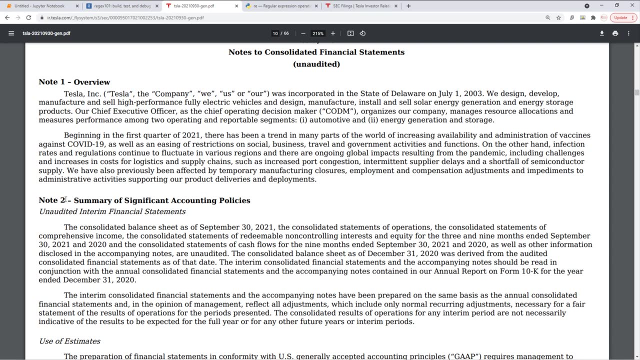 you will see the special tokens that you will be using in regular expression for the pattern matching. now for pattern matching. pattern matching, of course, you can use simple string match in python, but using regex is going to make your life much easier and we'll see that in. 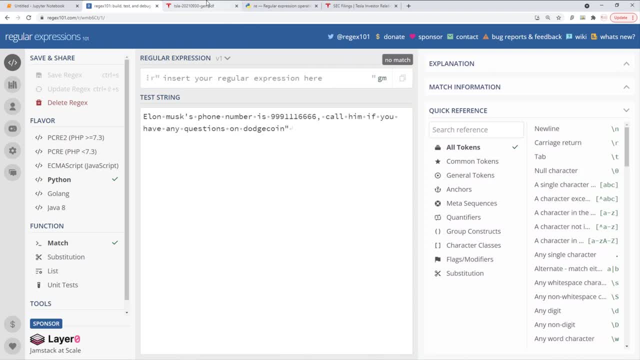 future videos seconds. let's say I have a very simple string. I mean I'm going to go to this notes section little later, but let's say just for net practice. let's say this is a simple string. I'm giving you Elon Musk number if you have any questions on dogecoin. by the way, this is a dummy. 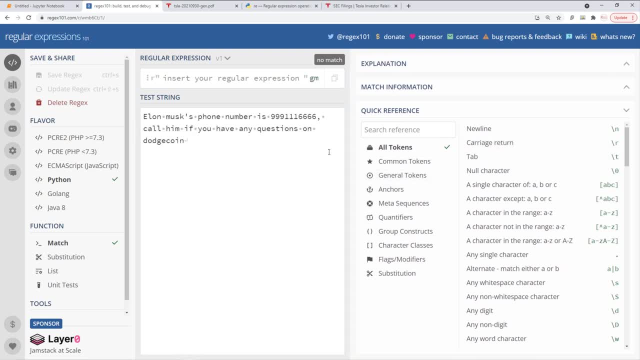 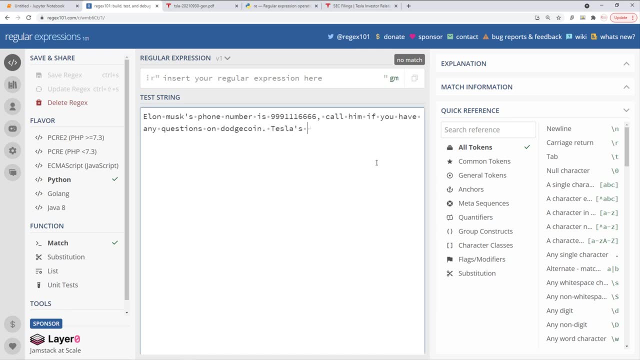 number, so don't even try. okay, here I want to extract a phone number. okay, from this number you can say: okay, Tesla's revenue is 100, whatever, it's not 40 billion really. but there are a couple of numbers in this text and you want to. 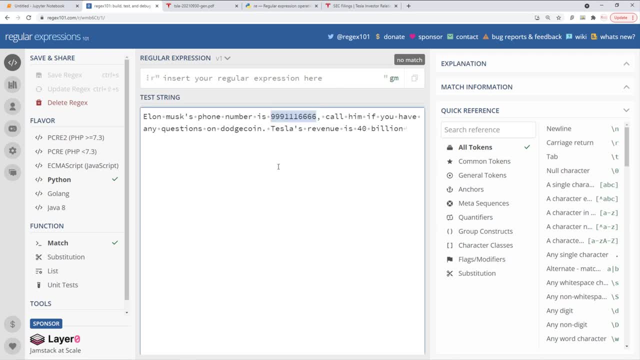 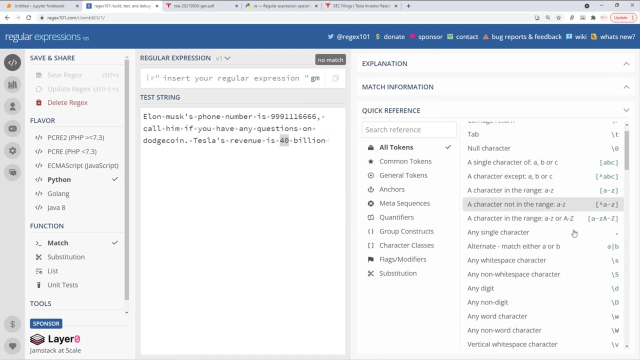 extract a phone number. a phone number is 10 digit. so whenever you say a 10 digit sequence or a pattern in your text, you want to extract that. now, this is 10 digit, but this is two digits. so you want to extract this, but not that. how do you do that? look at here slash d, so any digit is represented by 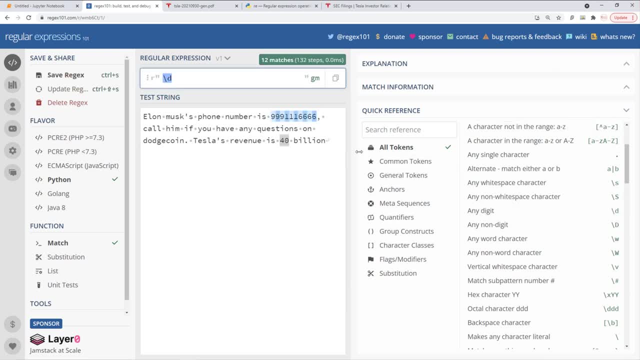 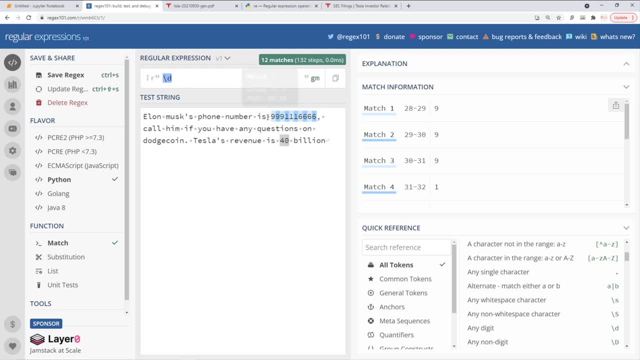 matches because it matches a single digit. how do I say that? I want to, you know, match multiple digits. well, you can do this. slash d now it will match two digits. see two consecutive digits: see 99, 91 and so on. how do I say three consecutive digits? well, see three consecutive digits: nine, nine, nine. 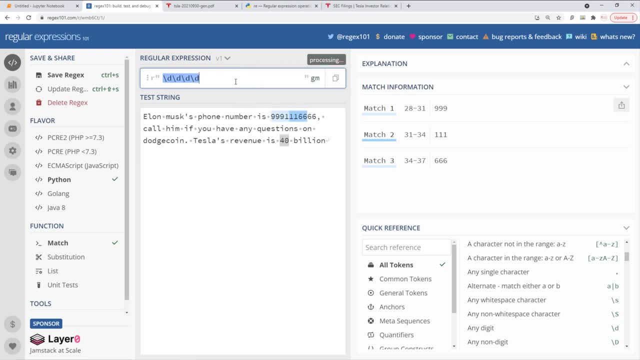 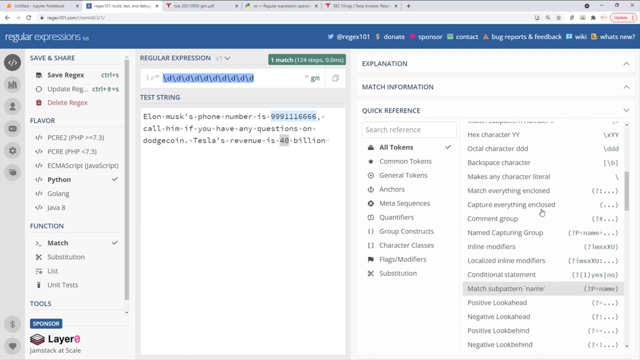 one, one, one, six, six, six, four consecutive digits: five, six, seven, eight, nine, ten. now this is one way you can extract phone number, because this regular expression is saying that extract any text which is 10 consecutive digits. there is a better way to write the same thing where: see in this help if you click on common tokens. 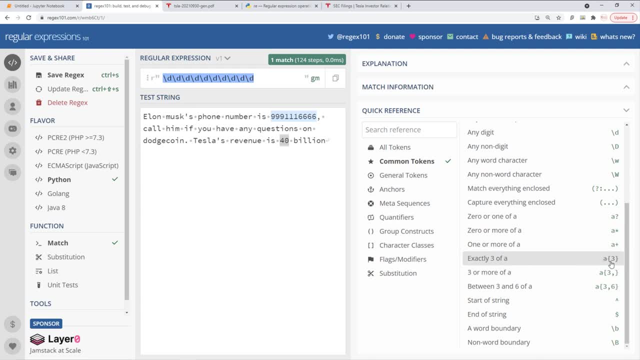 check this. it says exactly three occurrences of a. so I want to do same thing. I want to say exactly 10 occurrences of digits 0 to 9 and if you look at match information see it exactly match that. so this is how you use this tokens. what if I have a different number in a different format, sometimes in US? 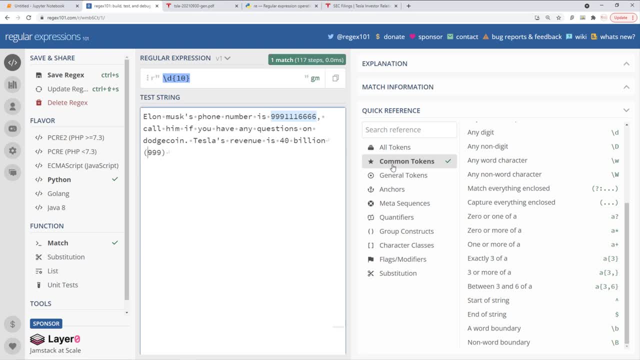 the numbers can be represented as like this: you know, laissez-là's is this. now, this number is in a little different format, but it's still a valid USA number. if you want to extract this as well as that, what do you do? okay, first, 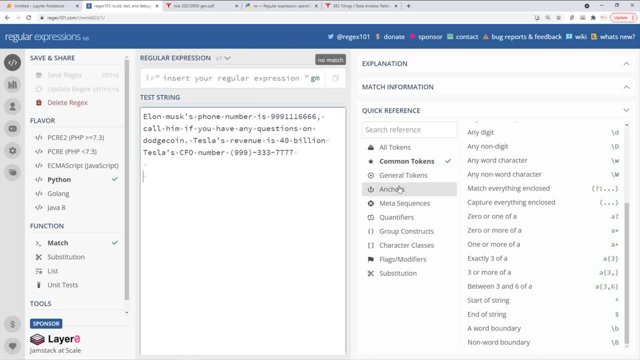 we know. okay, this expression, let me just put it here. this is the expression for this simple number. let's write a regular expression to extract this particular number. okay, in this number we have a bracket first. so whenever you want to do a match, let's see if i do do elon, see it is, it is matching that. 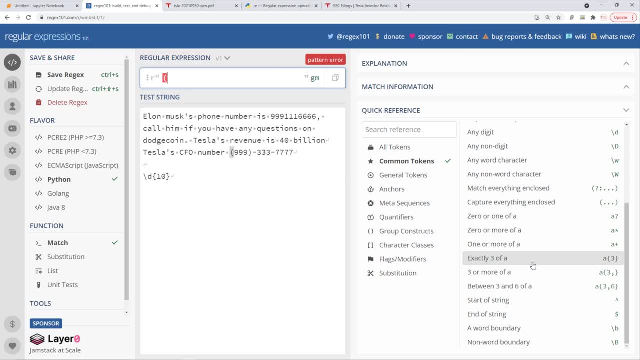 so i can do this and it will match that. but bracket has a special meaning. it's a special character. see bracket, let's see capture everything and close. so it has a different meaning. i will go there in a bit, but assume bracket is a special character and whenever you have special character. 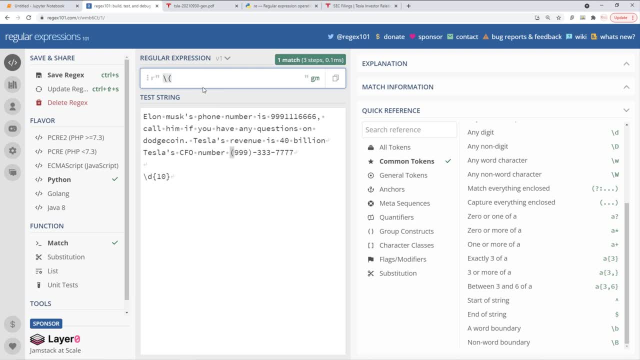 and if and if you want to do a literal match, you will put slash here. doing that will exactly match that. and then i have three digits, exactly three digits, and see if you have 10 digits, you do this. if you have three digits, you do that, cool. and then you have another bracket, but bracket again. 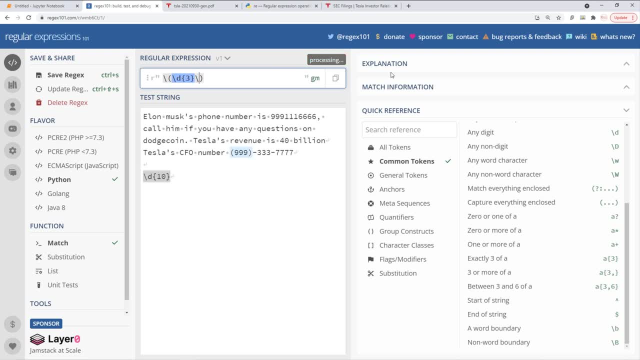 bracket is a special character, so you need to put slash here. see, this looks complex, but if you gradually build it it's not that complex. then you have hyphen, then you have exactly three digits, then hyphen, then exactly four digits. see, now it is matching this particular pattern pattern. 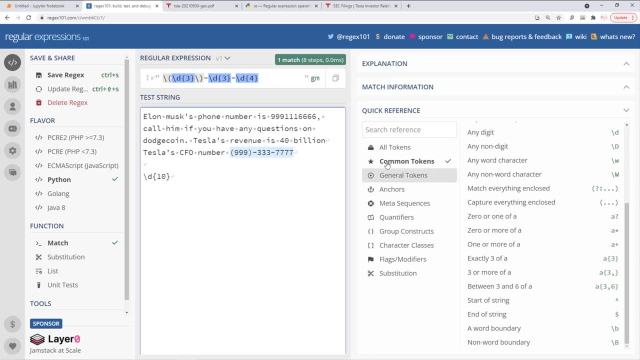 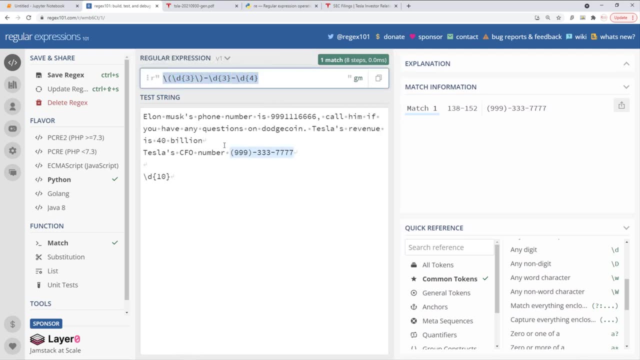 if you have anything less, it will not match. see, it is highlighting the character, so you can see it's, which means it is matching and you can see it here. so i want, so i have this regular expression for this number and this expression for that number. so how do i do? or i want either of these. 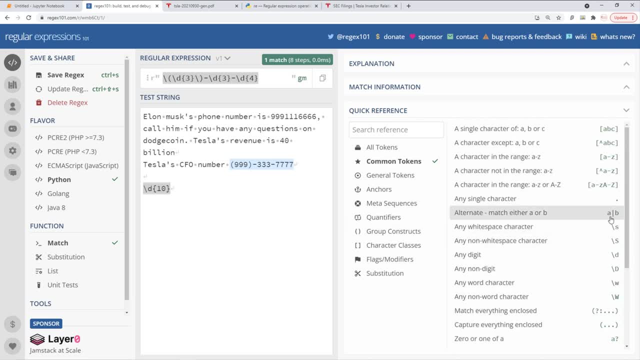 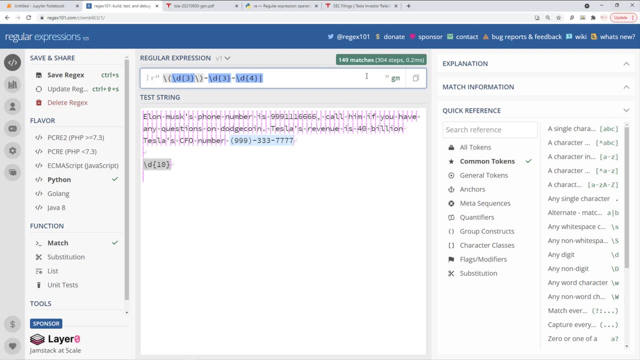 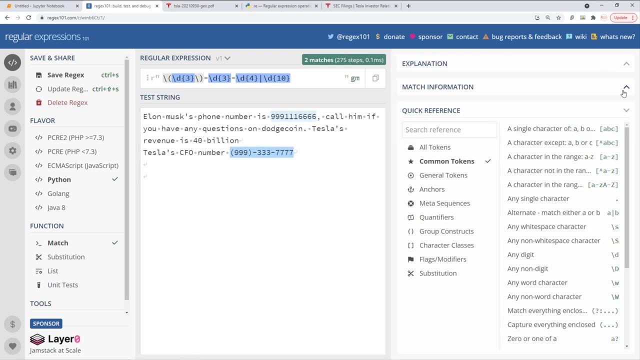 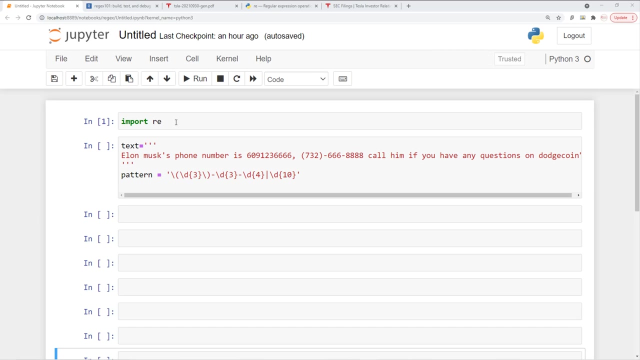 to be matching and for or. i have this character see a or b, so i can now do a or b. cool, see, now it is matching this number and that number. now let me do the same thing in python code. so in my jupyter notebook i have imported a module called re and that's what we use for regular expression. 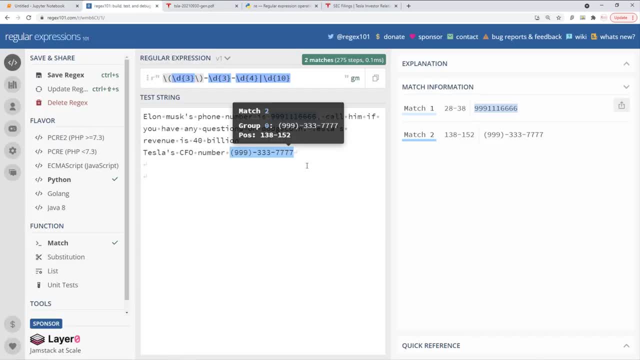 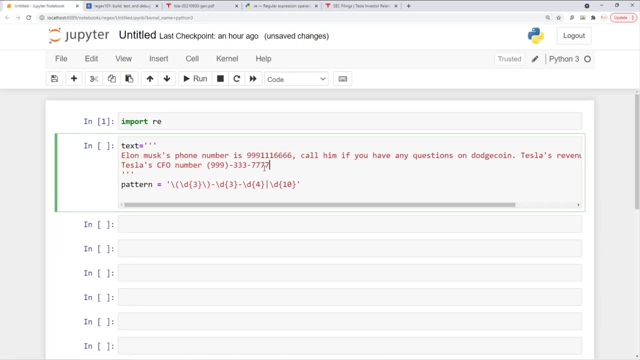 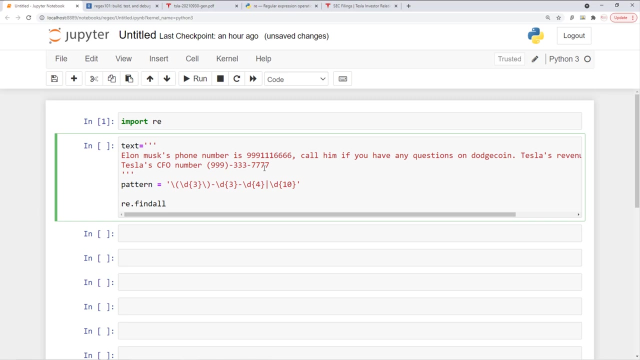 and i have that text here. okay, so what is my text? so my text, i'll just copy paste that text here. so my text is this, my pattern is this: and you will do: re dot, find all, find all, will find all your matches, you will supply your. 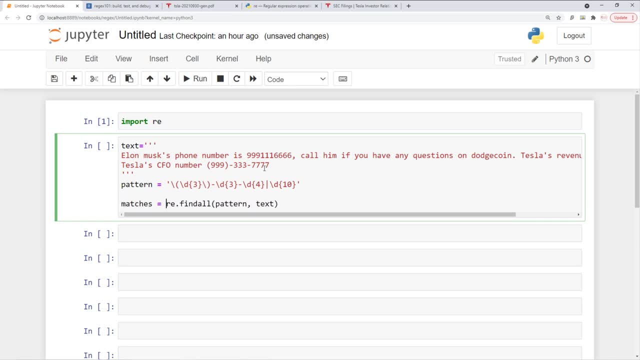 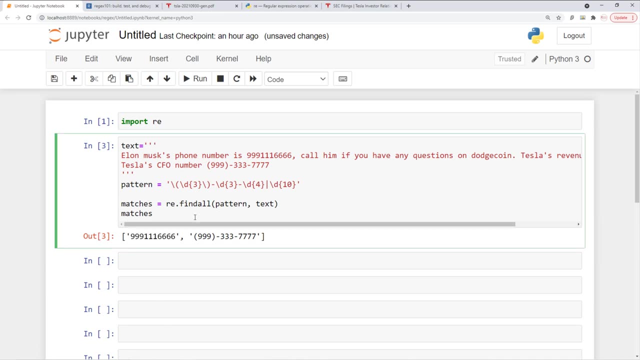 pattern here, then text here, and then you will say: matches. okay, see it, match both of this number. so this is a very effective way. now, if you want to write the same thing in a plain python without using regular expression, try it out. it's going to be much difficult. all right, awesome, now let's go. 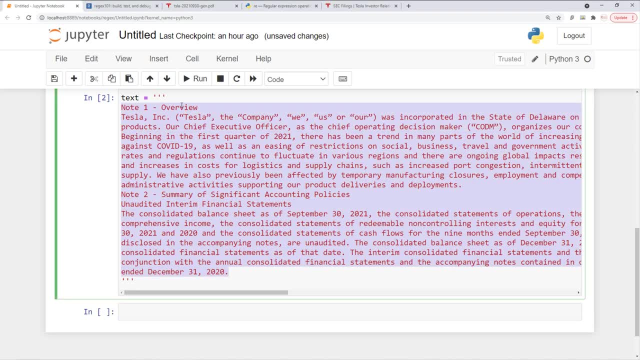 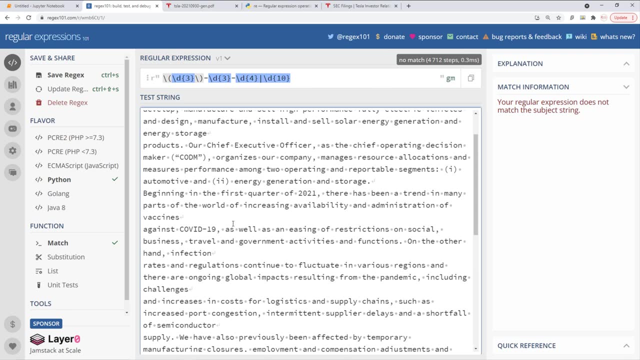 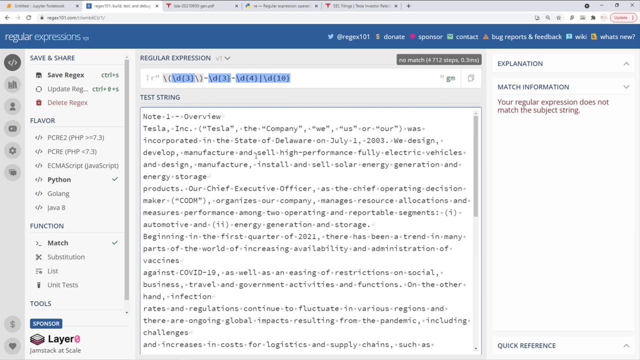 back to our main problem, which is extracting the note title. so i'm going to copy, paste this, paste this huge code block and again my goal is to extract note title which is overview and summary of significant accounting policies. so let's try this out. so to match note, you will say note, then there is space. 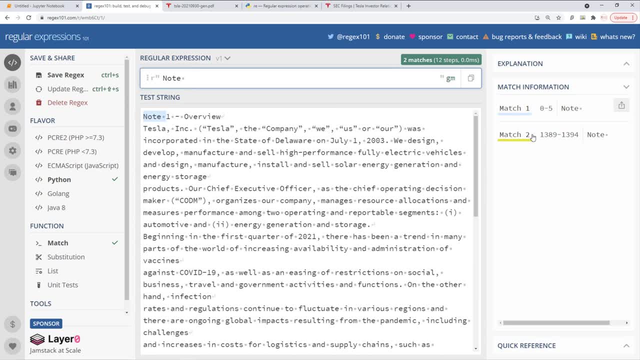 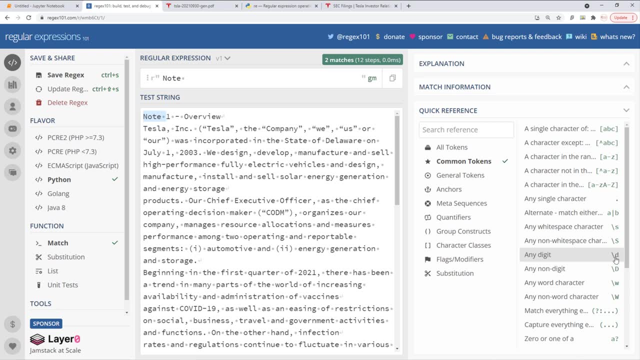 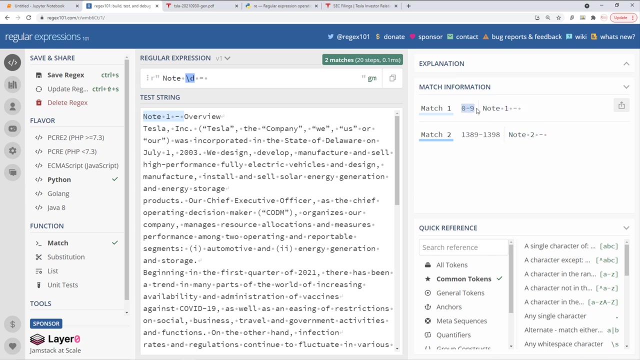 okay, and after that there could be any digit, one, two and so on, and you already know that we will find it. what do we use? well, we use here, see slash d. so you will do slash d, then space, then hyphen, then space. okay, so so far we matched note one and note two and you'll see the character range. 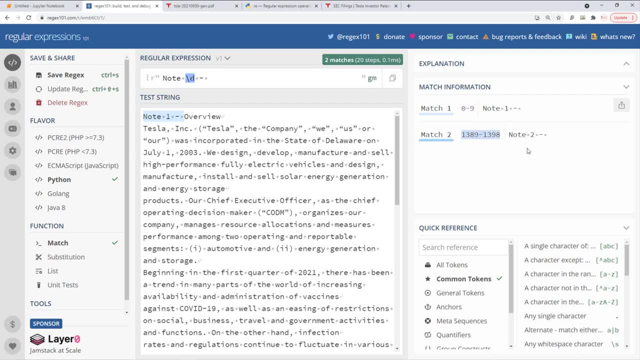 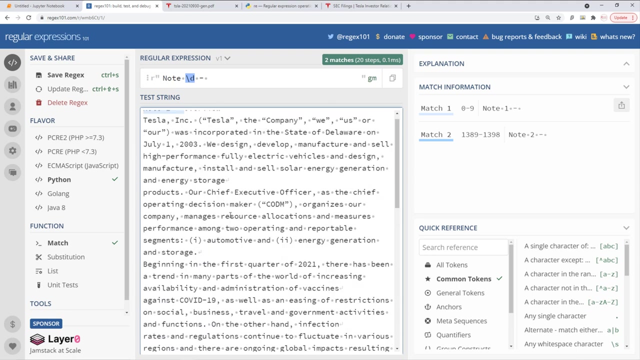 see zero, two nine character in my text block is one and this character range is not two. now think about it. you want to capture everything that starts from here till you find slash n. so slash n is a new line. so anything that comes in a way before you encounter slash n, which is a new line, you 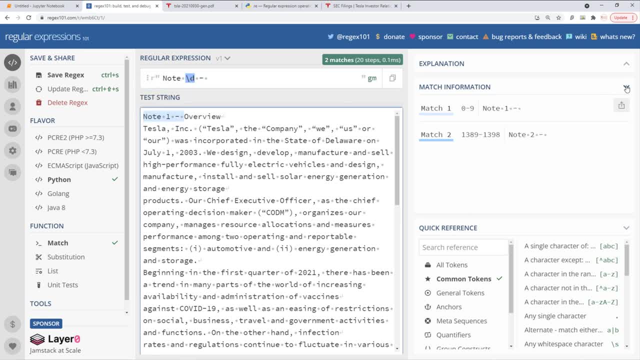 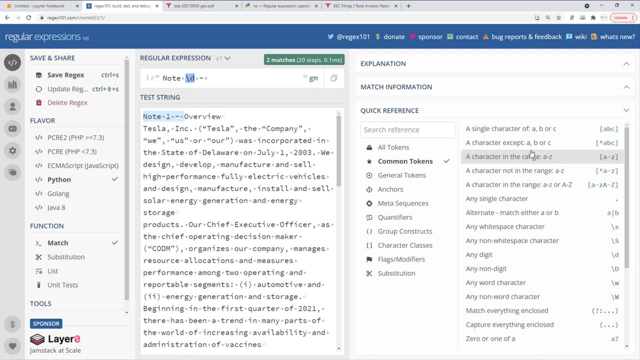 want to capture all of that. how do you say that in regular expression language: check this: any character except a, b or c. so when you want to say i want any character except this particular character, you will say this particular: um, you know this, this carriage return. so 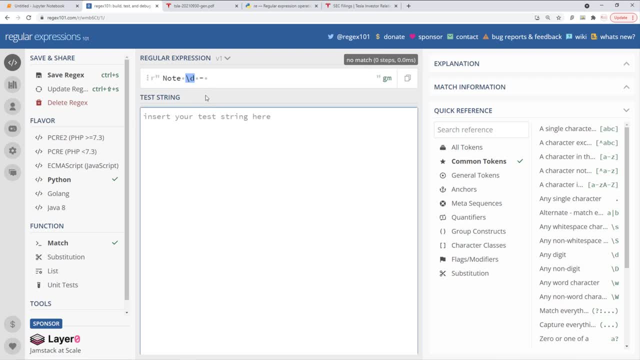 let me remove it and just just to make things simple, i will type something in. so let's say: i have these characters, you know, and now you want to say any character except this and that. so to do that, you will do this particular character and you will say: 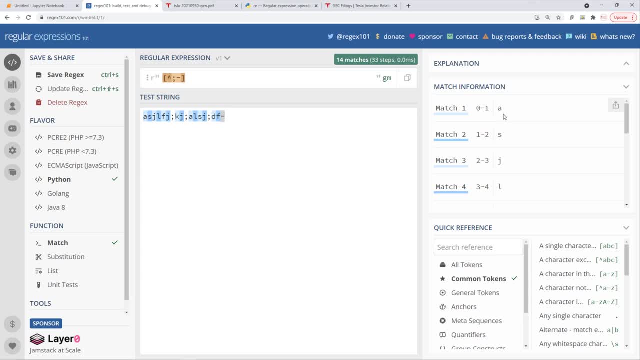 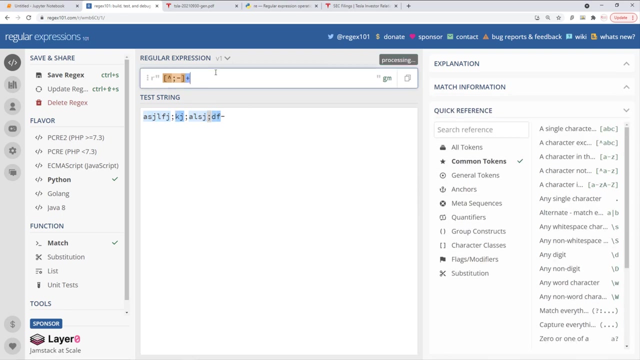 say so now. it matches all this character, a as J, LFL, whatever- but it did not match this character and that character, and if you want to do a sequence you can do plus as well. so when you do plus it is like one or more of those characters. so 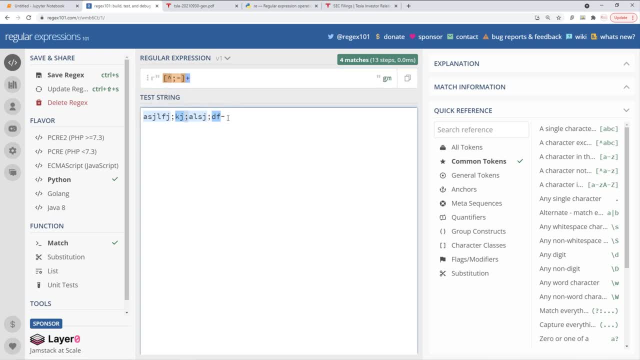 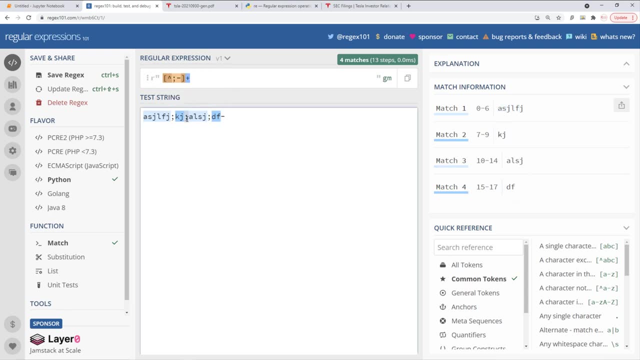 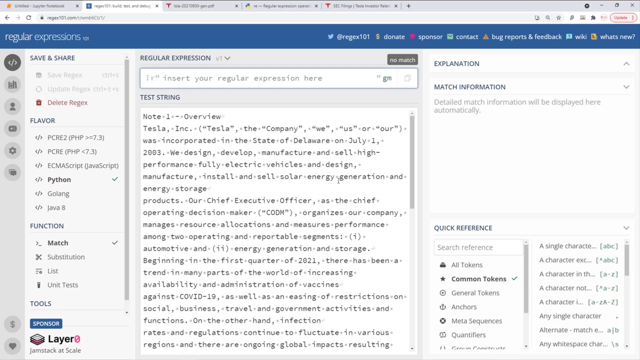 one or more of those characters, which is not semicolon and hyphen. so see, now look at match information. it match this, this, that, but it did not match semicolon and this. okay, we have back to our node example. sorry for back-and-forth, so not. then space this less D, note space and then slash T. then 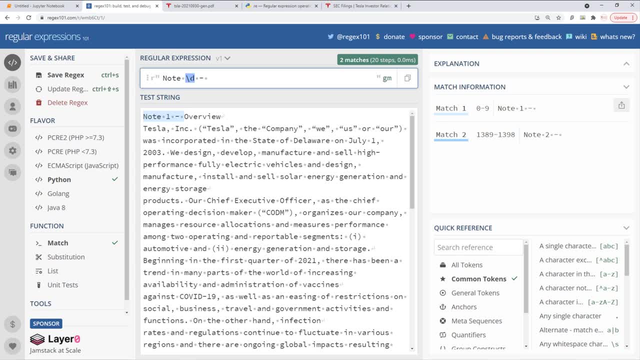 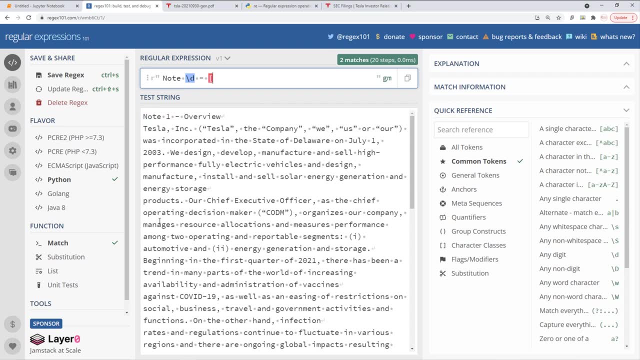 space, hyphen, space, now, any character except slash n. so you would do something like this: okay, so you're saying any character, but slash n. now, when you do that, see, it is matching. oh, it is matching O here, it is matching S here. but I want that. 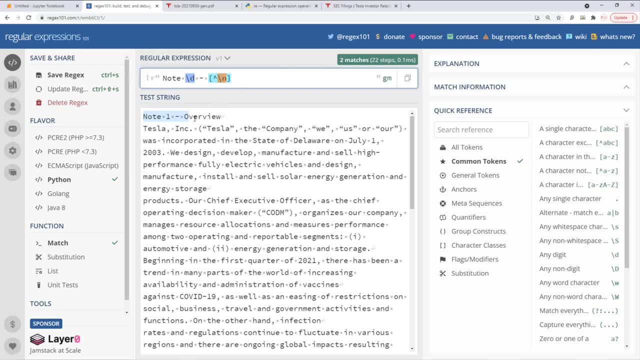 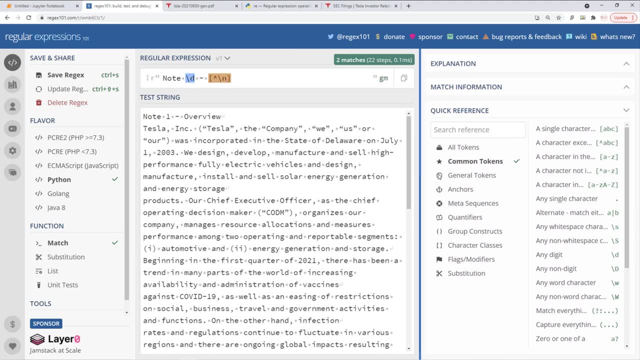 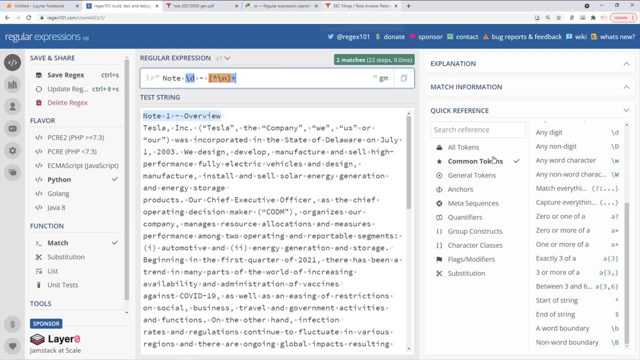 repetition. you know I want any character except slash n and a character sequence. I don't want only one character. and when you want to match one or more of those characters, you will say plus, C, plus. so I will say plus if you want to match 0 or 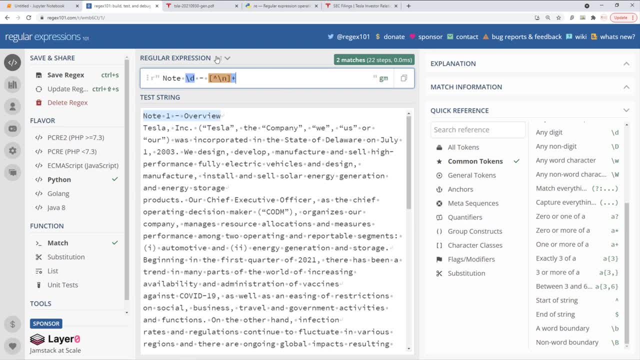 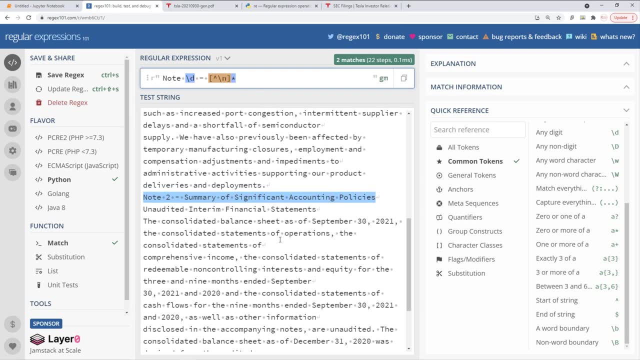 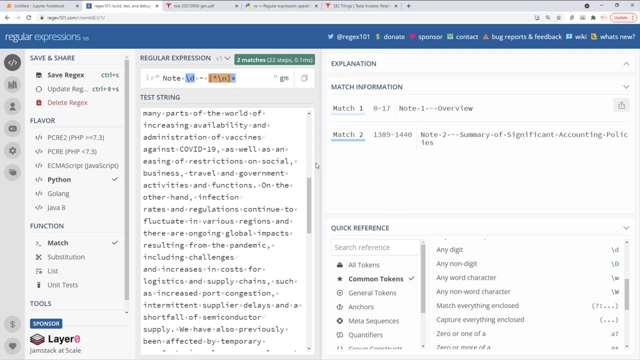 more of character a, you will do star. so the right thing if you have a blank title and if you still want to get that, the right thing to do here will be star. okay, hooray, look at this. i have my title. see overview. summary of significant 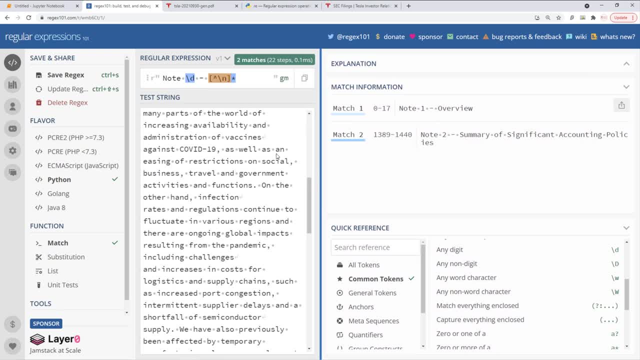 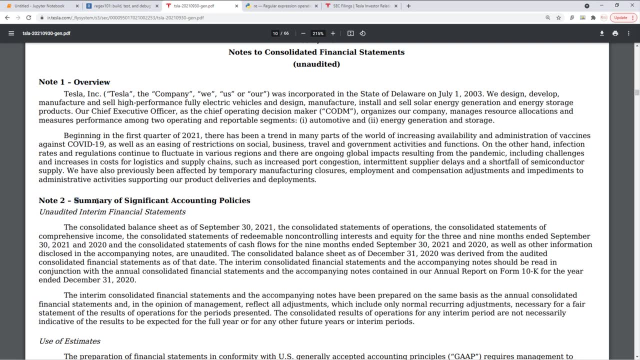 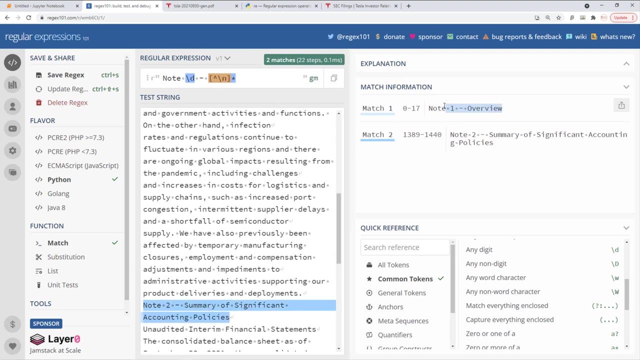 policies. so i matched those two. but i want only title. so my title is: see, my title here is overview. i want to extract overview and then summary of significant policies, so to match those titles. you know, see, there are two things. one is match information, which is the which is short of like. 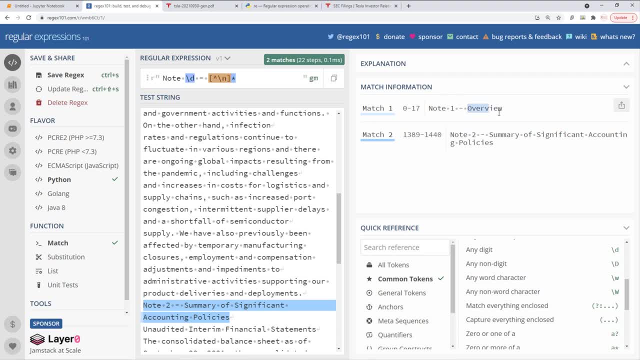 a string match, but you want to extract only a portion of that match. so the portion of that match is anything that start after this space- see after this space. so you will put a bracket here. when you put a bracket, what happens is it will perform a match, but from that match it will capture everything that is within those 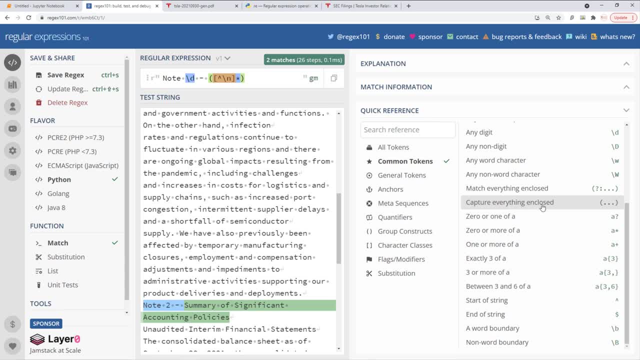 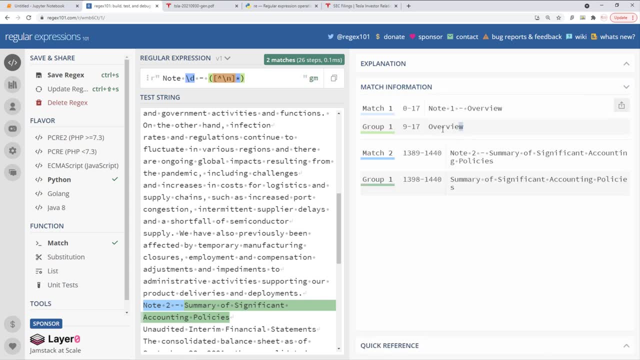 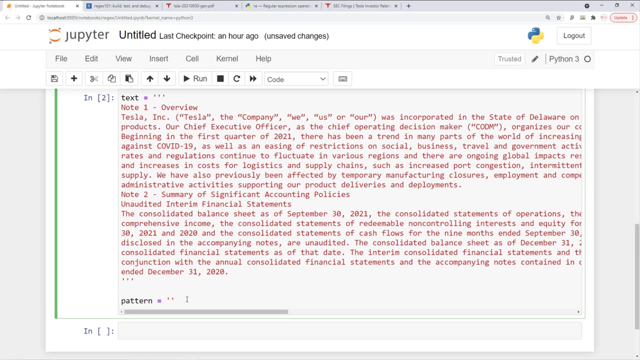 brackets. so what is within those brackets? see here, capture everything, and close meaning bracket, and after that, inside those brackets, whatever there is, it will capture all of that. so now i'm going to just copy paste this pattern here in a pattern variable and i will say: read the. 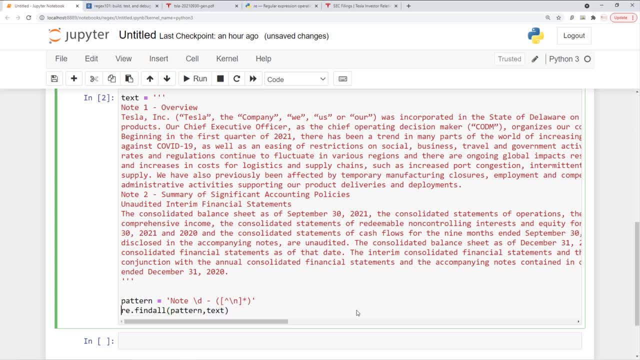 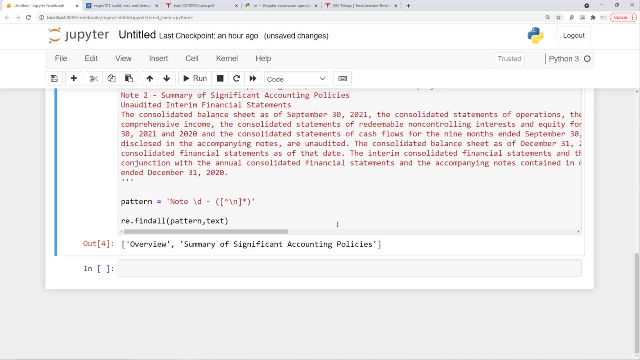 find all pattern text and see now what i find is i have overview and summary of significant accounting policies. see, when you look at the expression itself, it looks difficult. i mean to me it looks difficult. but if you build it slowly, step by step, it is not that hard. 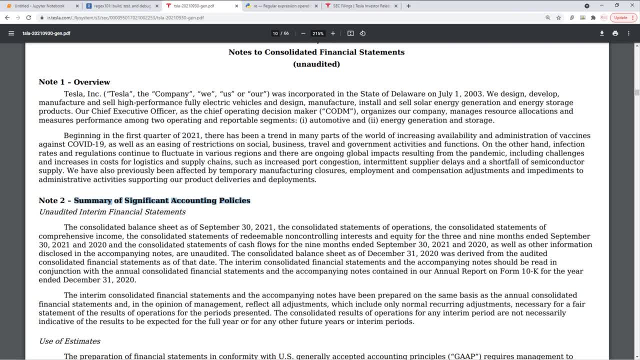 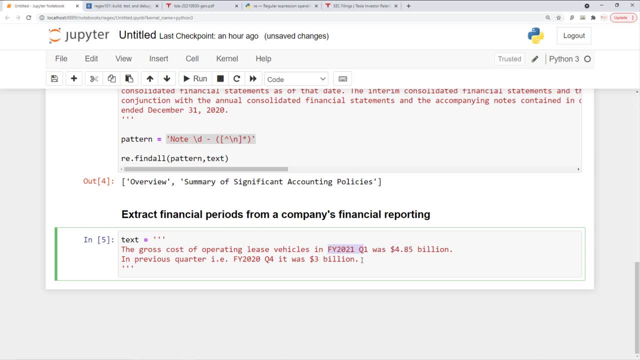 now the next thing i'm going to do is i took some text block from this document and i will extract the company financial periods. so company financial period is anything that starts with fy, after that there is a year and then there is a space, and then there will be quarters, so it could be q1, q2, q3, q4. 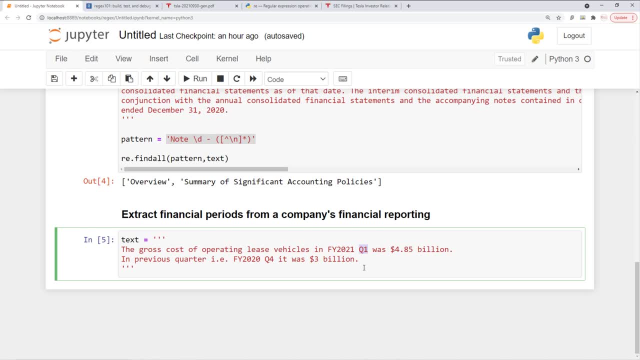 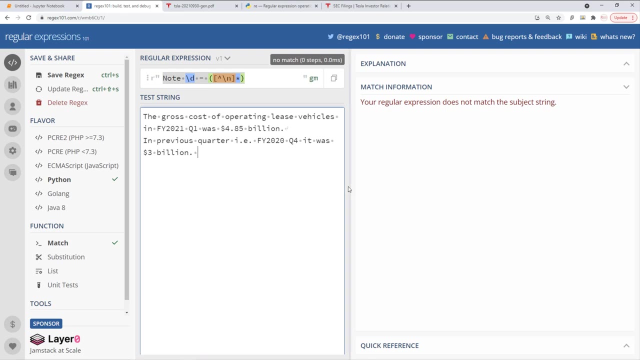 one quarter is three months. there cannot be q5, so i want to extract from this tags fy 2021- q1 and fy 2020- 4.. so let's do this in our test pad first, as usual. so I'm just going to copy paste this thing here and 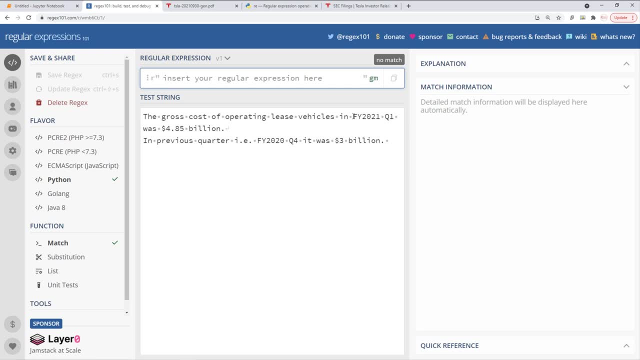 remove this, okay. so what is the pattern? pattern is: it always starts with FY, so let's put FY first, then there should be four digits, exactly four digits. how do you do that? you already know that slash D four: see four digits. so now my match one is this. match two is this: after that there is a space. see this dot means. 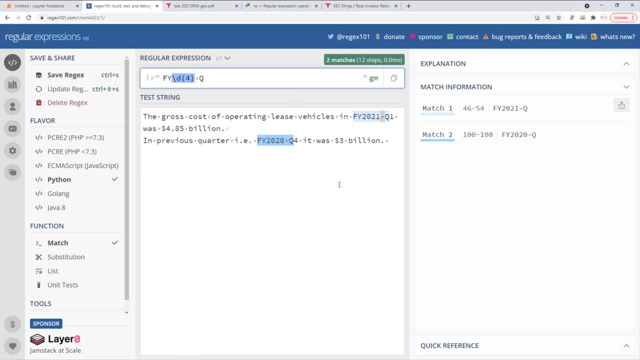 space, so space, and then there is Q. and then see, now I cannot do slash D. see, doing slash D matches this. but it will match things like this to Q5. Q5 is not a valid financial quarter. the number has to be either one, two, three or four. 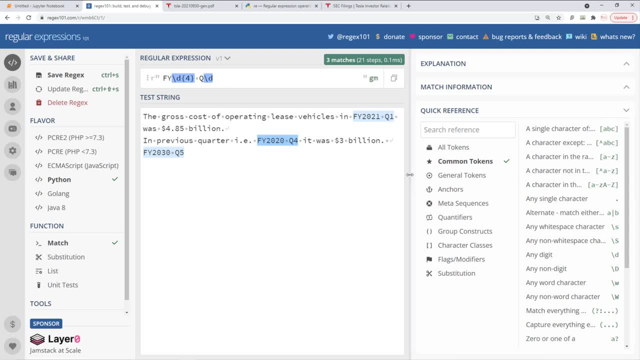 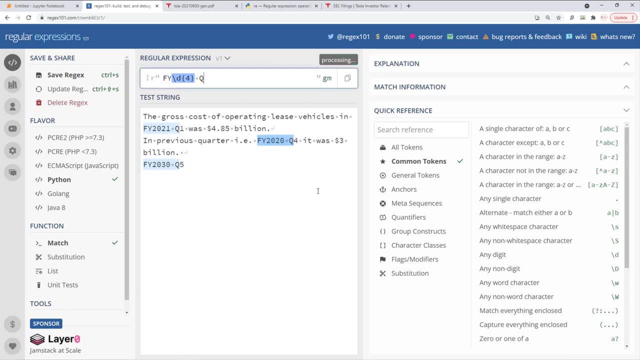 and if you look at this help, it says a single case. then Q5 is valid financial quarter and then there is a three numbers after that. there is to be either one, two, three or four. and if you look at this help, it says a single case character of this. so if you want to explicitly mention your choices, what you 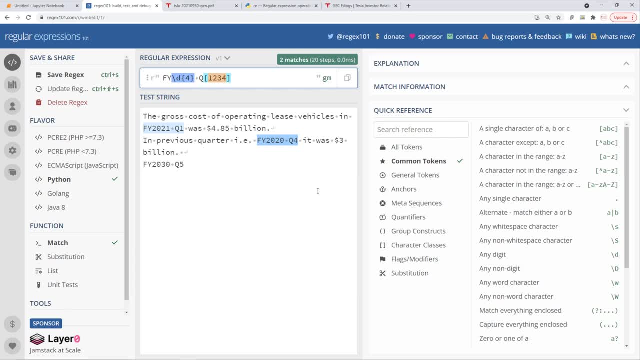 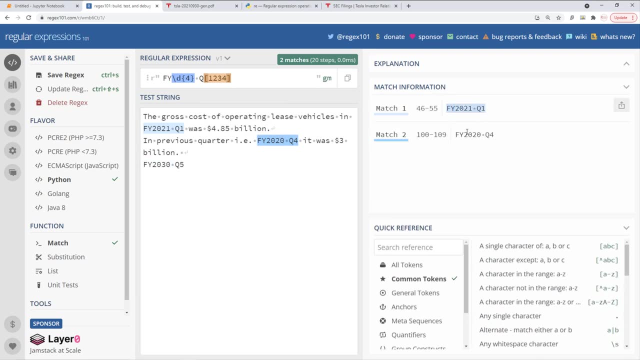 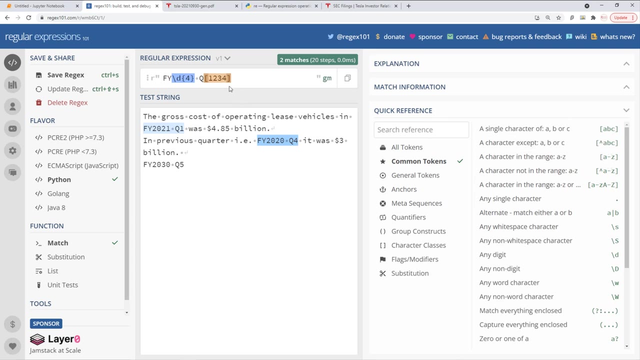 can do is 1, 2, 3, 4. so match either 1 or 2 or 3 or 4 and see it matched these two, but this did not match. okay, you can see this and match information. this is one way. the other way is this: see, you can specify a range, so any number in range. 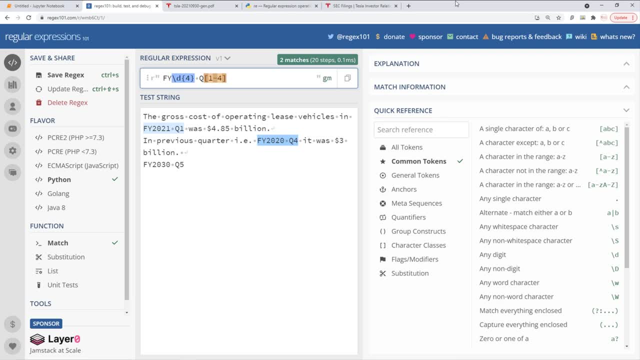 1, 2, 4, any number in range- 1, 2, 4. friends, this is not hard. stay on this. I'm telling you this is easy. see, think about it. take a pause. think about this: 1, 2, 4 and it matched that. see, this is super easy, it's not hard at all, and I'm going. 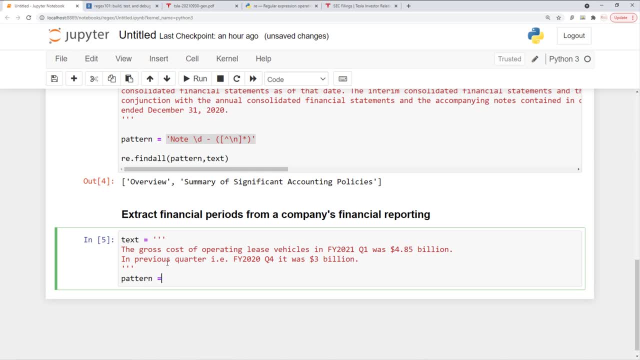 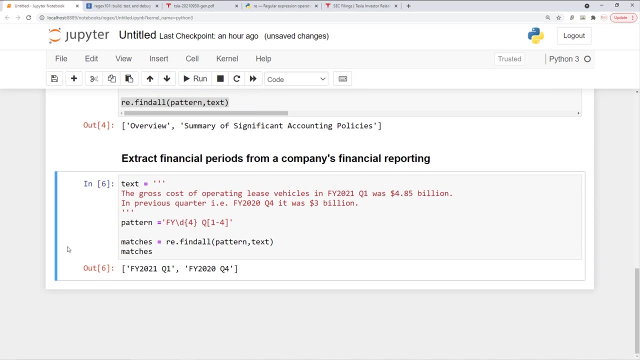 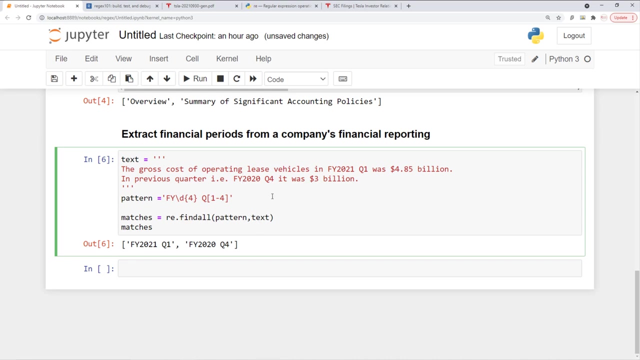 to now copy paste this pattern here, and then, you know, just copy paste. and right now I'm going to paste this pattern here, and then, you know, just copy paste. and, by the way, you can store this in a variable for matches and print matches instead. see it matched, both of this. now, what if there is a? you know this case? 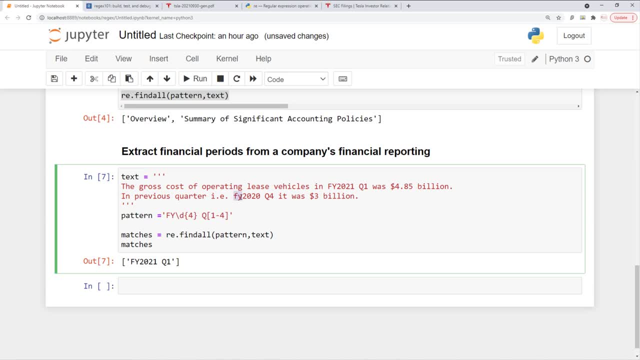 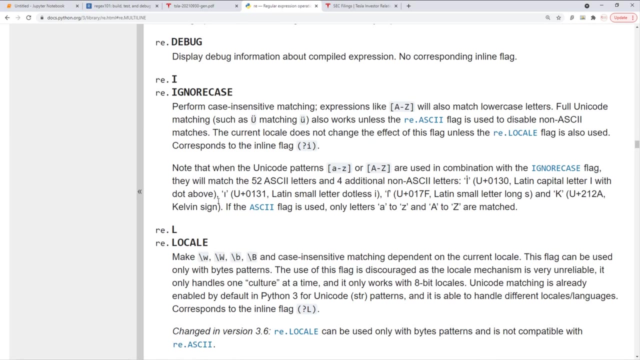 sensitive. f5, for example, says the lowercase and if you want to take a lowercase, that there are flags that you can match the flags is equal to RE dot and if you read the documentation you can just say python, rag X flags. you will find all these flags and i'm going to use ignore case. see re dot, ignore case. 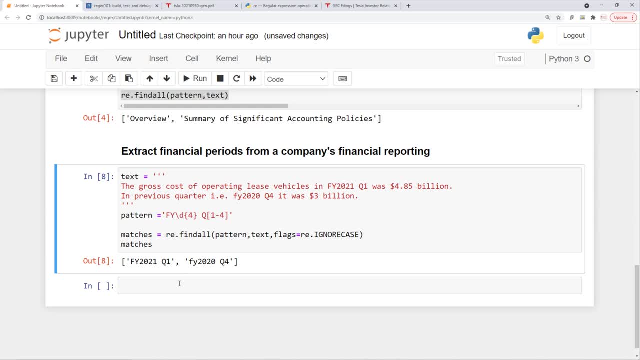 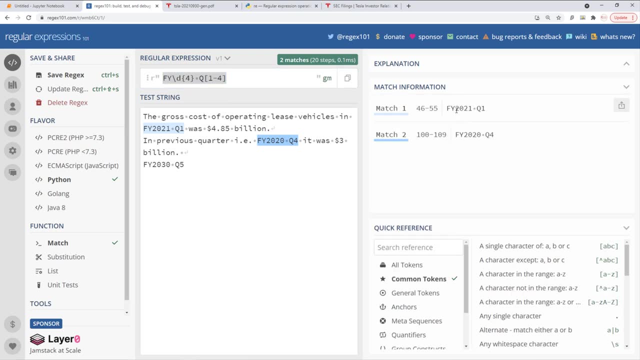 and when you ignore case, it will match capital fy as well as small fy. now, when i extract this financial information, sometimes i want to extract only 2021 q1 and 2020 q4. i don't want to put fy. okay, one option is: okay, i extract this and then i remove fi character explicitly, or you can be a 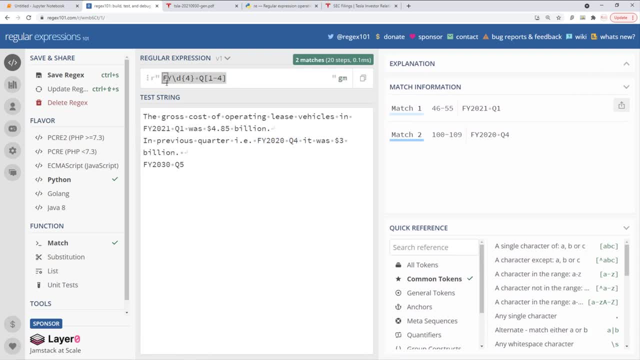 little smarter kid and you can use this bracket. we already saw that in regular expression there is something called match and after you match something, you can extract sub the part of that match using a bracket. so part of that match using a bracket would be this. so i put a bracket here. 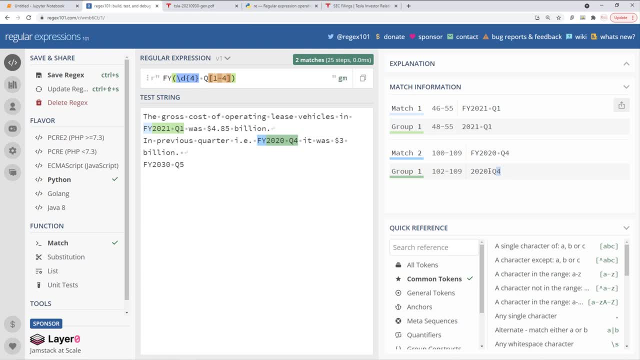 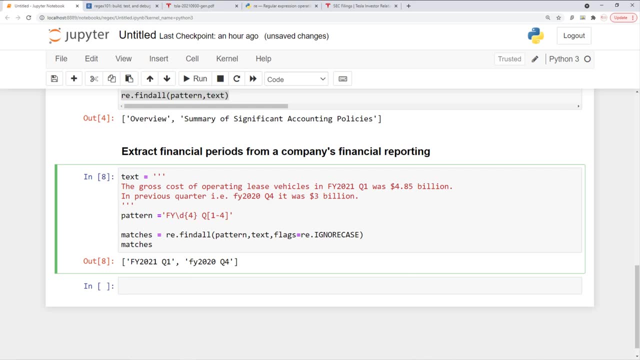 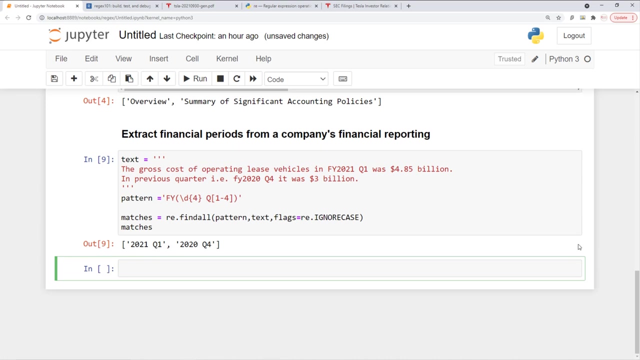 and when i put a bracket: see, my group one is 2020, q1, q4. so now let me uh, extract that particular thing here. well, i can just put a bracket here and you will see. now i have only the information that i need now, instead of financial number. let's extract. 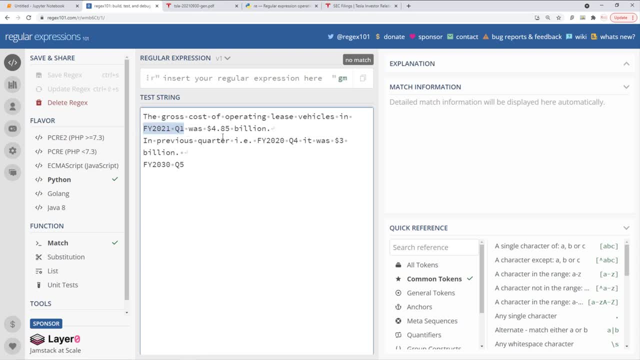 the actual values, you know, instead of financial, basically periods, we are extracting the actual values for those periods. so which was 4.85 billion and 3 billion. how do you do that? well, see, i can have n number of numbers, you know. i can have things like: tesla's employee count is, let's say, 5400. 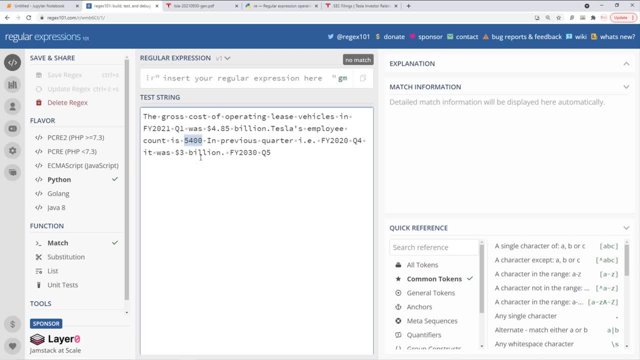 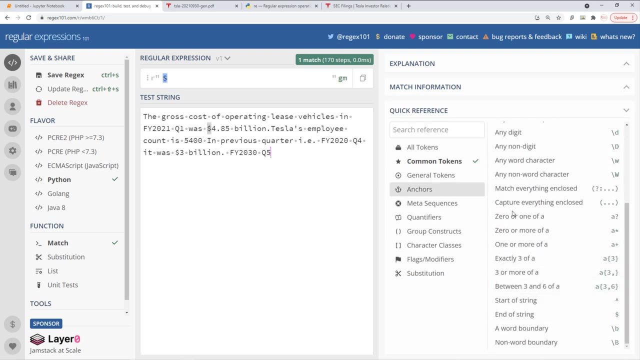 so when i extract those numbers i want to extract. i don't want to extract this, i want to extract anything that starts with dollar. so how about we put a dollar sign? well, if you put a dollar sign, again, dollar is a special character. see, dollar means end of the string, so it matched this thing. 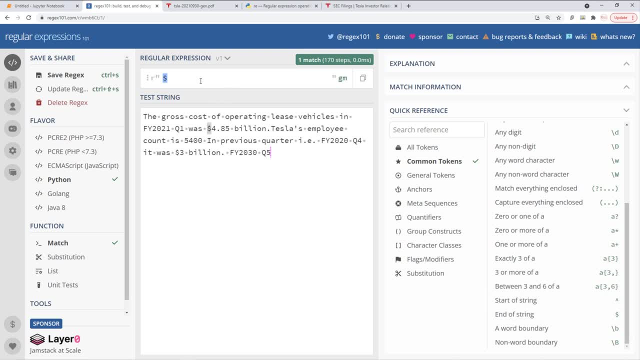 i don't want that actually. so for that reason, what we will do is this: we will put slash. so when you put a slash, it is an escape sequence. and now you are doing a literal match. literal match meaning you are not using dollar in a special way. your, if you have a dollar in your actual string, you. 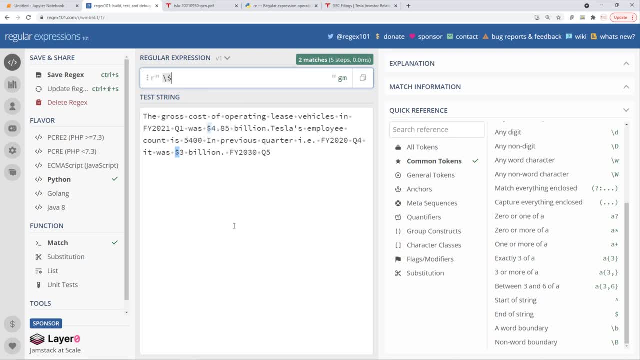 are doing that match and it found these two matches. after that you want to say any digits, so any digit is slash d. okay, but see, when you do that it is matching this. i can do any digit again, but now it did not match because there is this decimal. 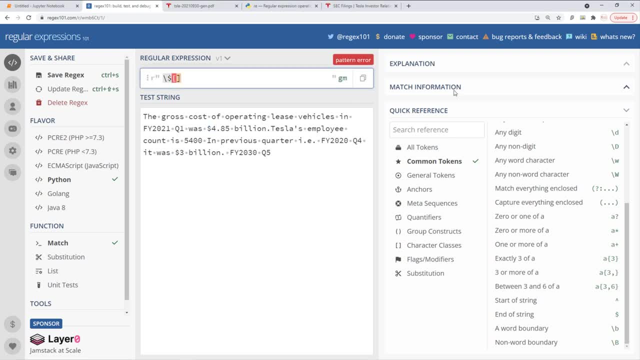 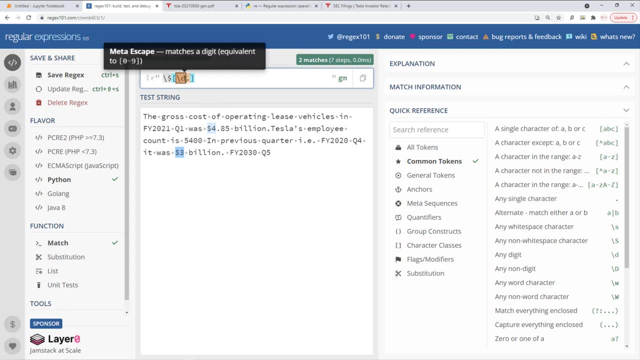 so instead i can do something like this: you know any digit and then decimal. now decimal again. dot is again a special character and you need to put slash here. and when you say plus, see, doing plus will match one or more character. if you do just this, it will match only first. 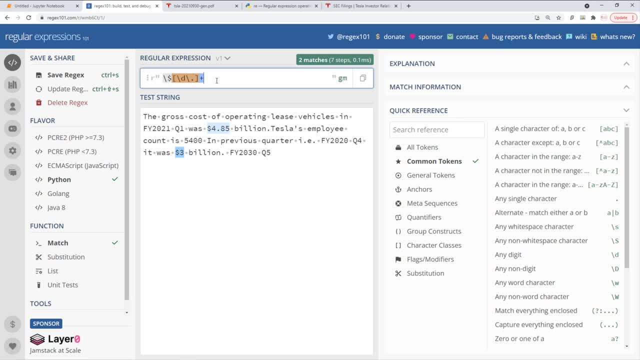 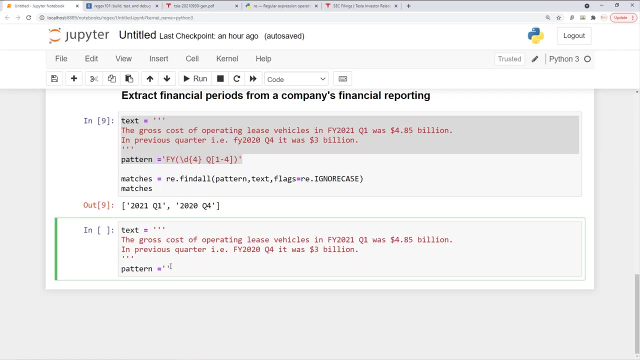 character. you want to say: match all the repeating characters until you find space or something. you so any digit or dot match that cool. you can also do something like zero to nine. zero to nine again means the same thing: any digit. okay, see here a character in this range. so i am going to now put this here and 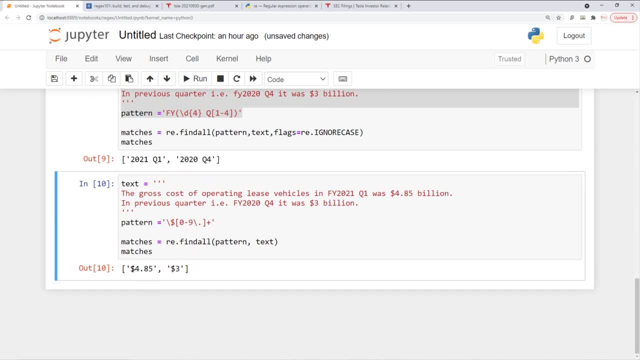 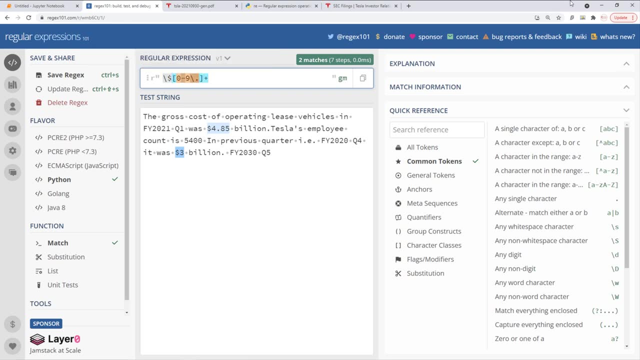 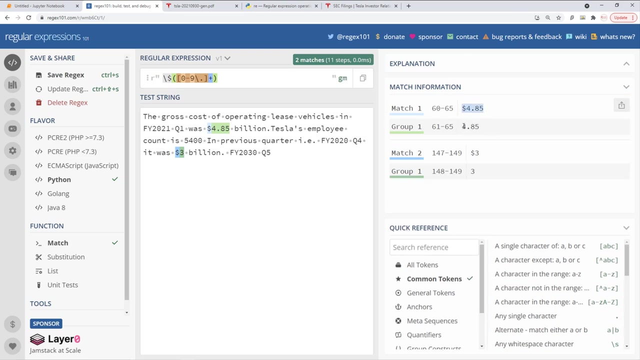 see it match this and once again you don't want to have dollar sign in your end result. so for capturing group you can do bracket. when you do bracket, see in the match information: match is dollar 4.85 but the group is 4.8503 so it removed dollar. so whenever you put something in bracket the group will have. 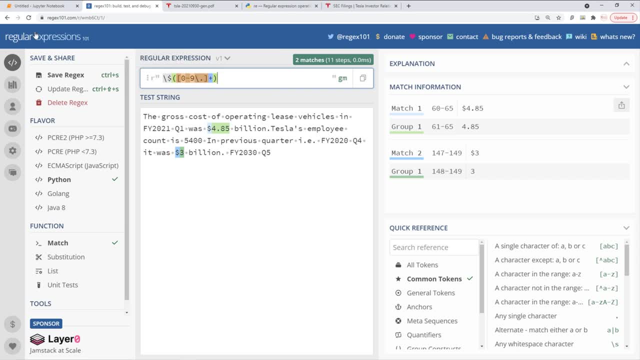 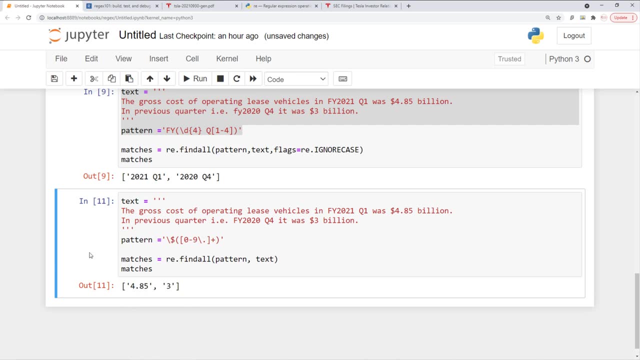 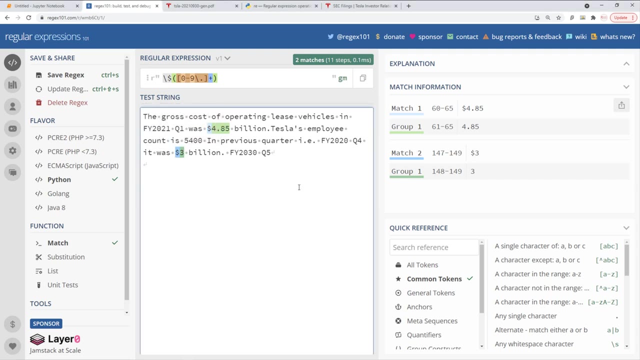 the content inside those brackets. only it will not include this dollar sign, so i will do bracket here and see those dollar signs are gone. now let's take little difficult task, which is i want to extract both the financial periods, so fy 2021- q1 and also 4.85, you see. so there should be financial period which says fy 2021- q1 is this and 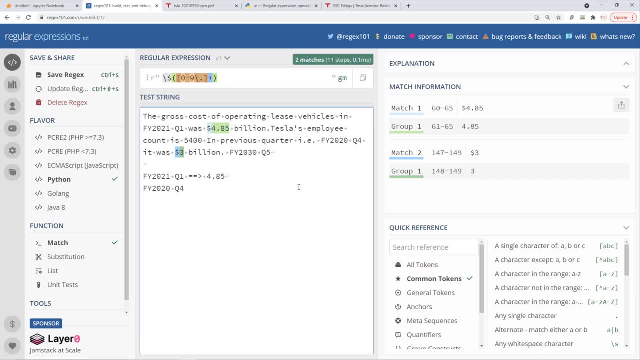 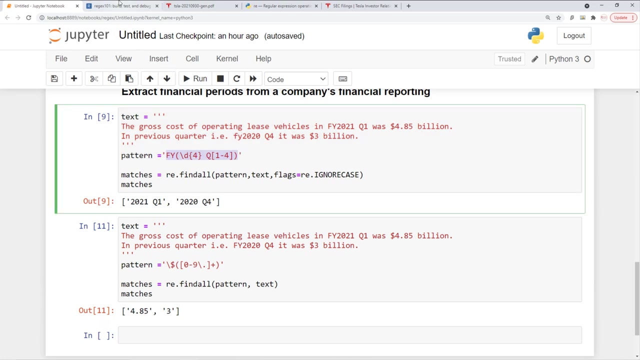 fy 2020 q4 is 3 billion, so i want to extract both of it. how do i do that? well, first you will write an expression to: to extract the financial period. okay, for financial period. what was our expression? it was this, right, so i will just copy paste that. okay now. 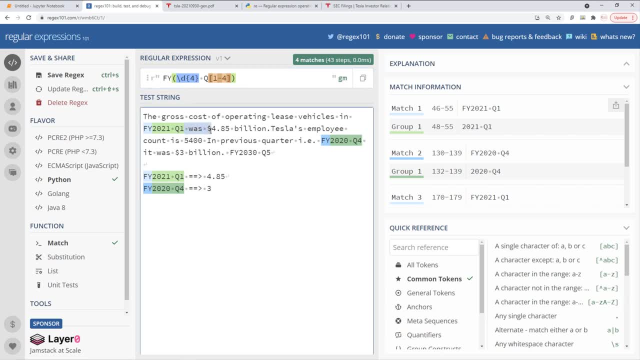 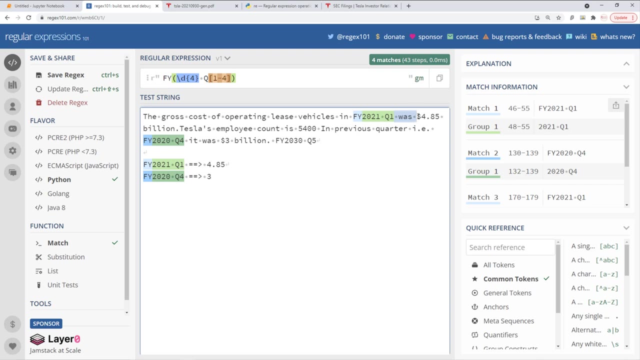 after i have my financial period, there could be you know n number of characters and then there will be a dollar sign. so my pattern is this: after my financial period, any character but dollar. so how do you do any character, any repeated character except dollar. how do you do that? well, you use 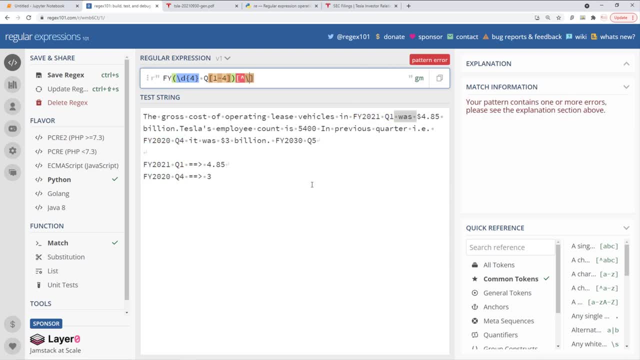 this one, right? if you already solved the question, then it's clear right after you've done that. so a previously any character, but dollar is this okay. so this is saying we are putting this slash because dollar is a special character, but this is really dollar and this will say any character, and this bracket is just a syntax. and 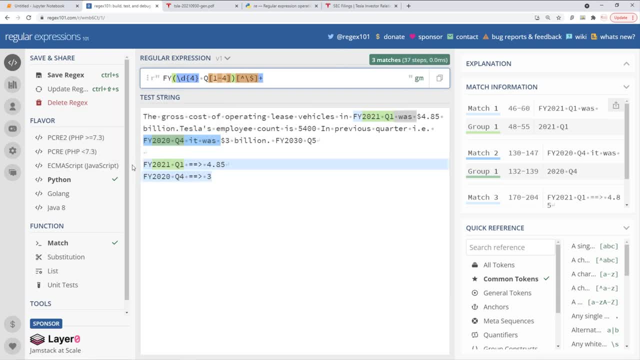 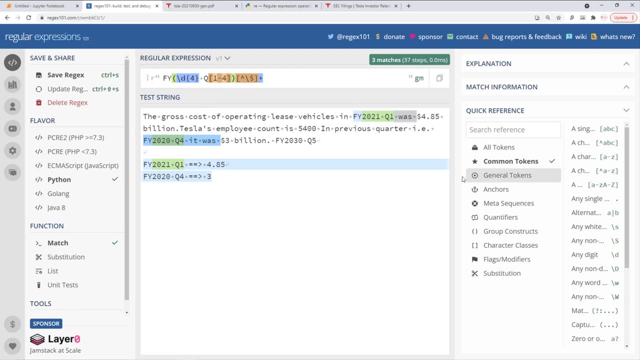 you will say: plus, plus means a repetition, you know. okay, now let me just make this little bigger here, okay. so we are going from here and we are going all the way here after you find dollar. so dollar is what slash dollar. so see, go friends, go slowly. this is not complex. I'm telling you: go slowly, don't get. 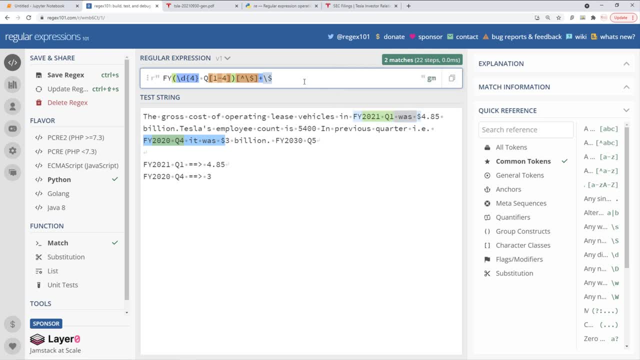 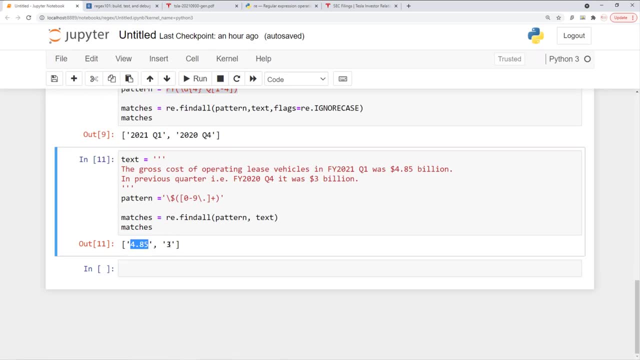 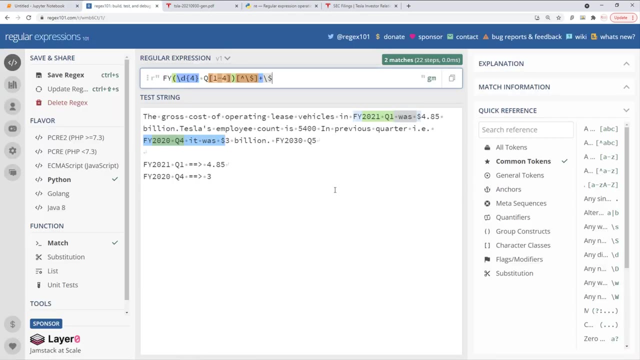 confused focus: slash dollar. so slash dollar is matching this. after that, you know what is the expression for. you know what is the expression for. you know what is the expression for matching this number? where expression is this? so I'm just going to copy paste. see, we are building these blogs one by one and just doing copy paste. okay, dollar. 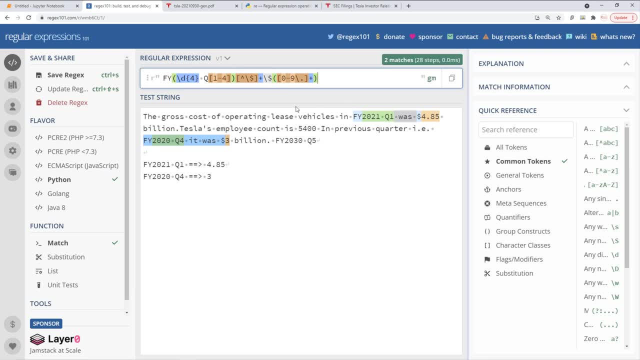 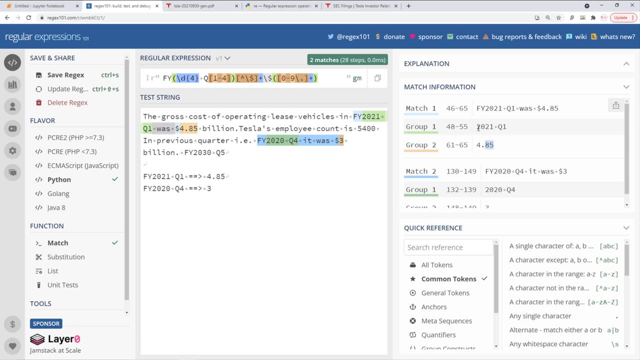 ID more cool and then you are putting that in the bracket. so, as a result, what happened was see. group one is this, group two is this. so now I'm saying: 2021 q1 number is four point eighty five. 2020 q4 is number three. so I can now. 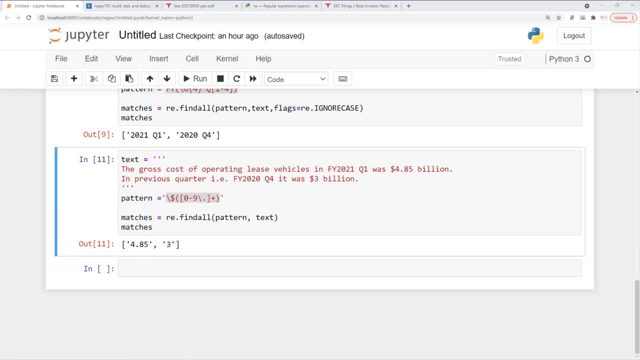 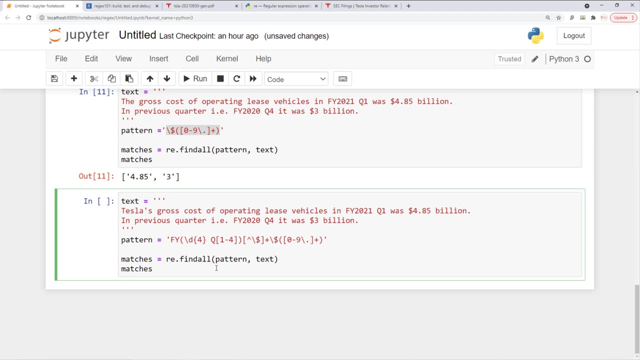 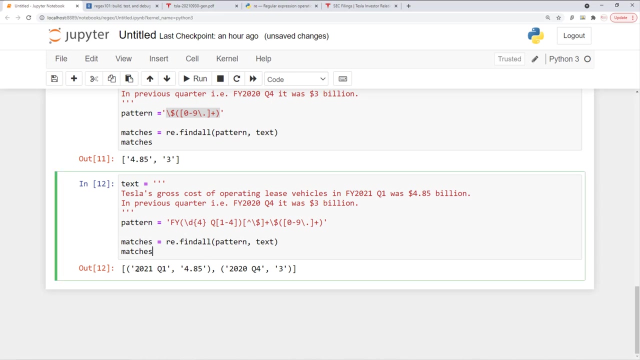 copy paste this particular thing here. see, I copy-paste it. that's that thing. and now matches: is this, it's this a couple? and this is awesome. now I'm saying 2021, Q 1 number, is this 20, 2024 number? is that other than find all? there is a method called search. okay, and we'll 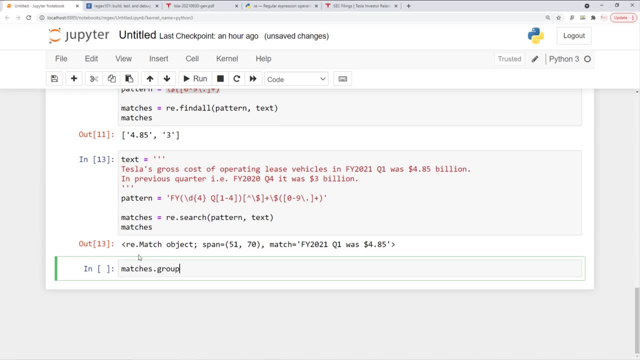 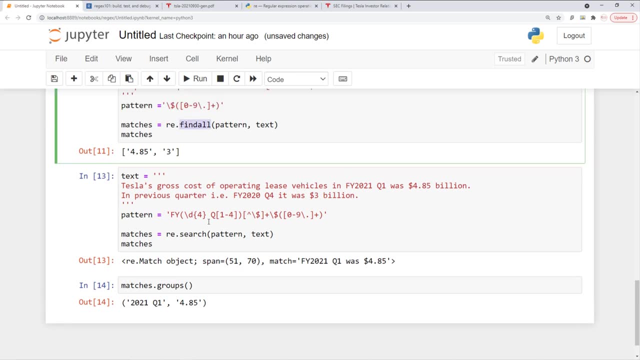 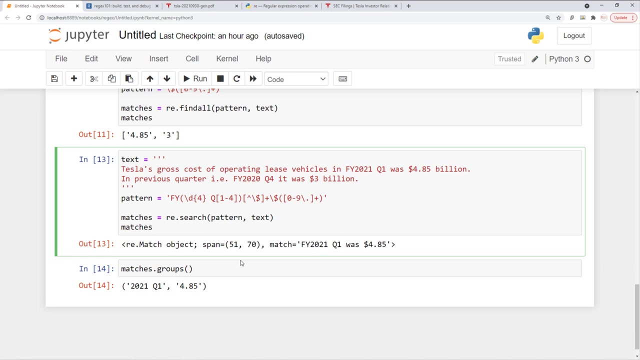 let's see what happens. the search has a different response where you have to do matchesgroups, but here it will search for the first occurrence, whereas the find all method will find all the occurrence. so that is a difference. all right, so that's all i had for this tutorial. now let's move.